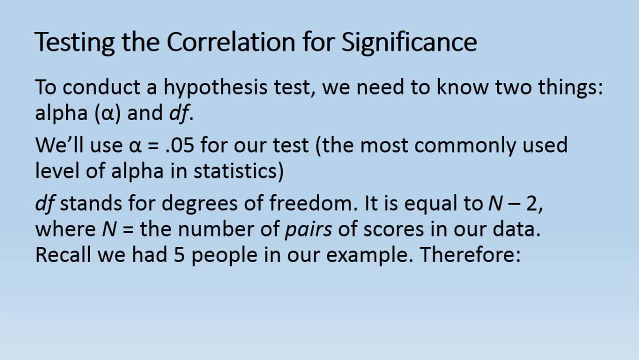 df stands for degrees of freedom. It is equal to n-2,, where n is equal to the number of pairs of scores. in our data Recall we had 5 people in our example, or 5 pairs of scores. Therefore, the df is equal to 5-2, or 3.. 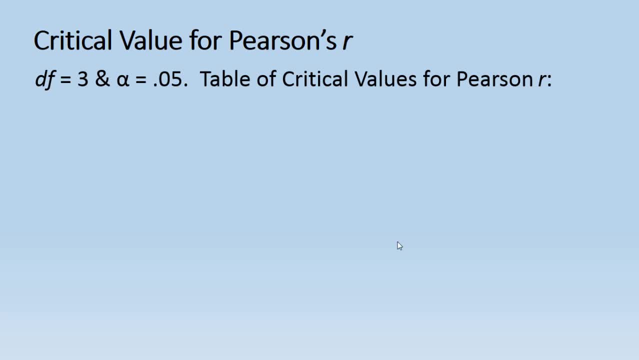 So once again, we have df of 3 and alpha of 0.05.. Now what we need to do is find the critical value for this test, And here's a snapshot of a table of critical values for Pearson's R, Remember alpha of 0.05, so we're going to work in this column. 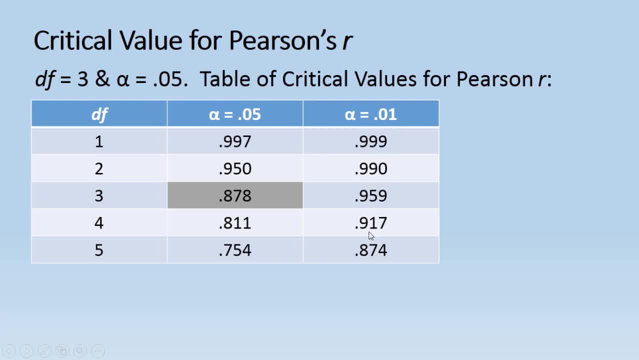 The second most common level of alpha is 0.01,, so I showed it here as well for those who are interested. But we're using 0.05,, which is the most commonly used level of alpha, And our df is 3.. 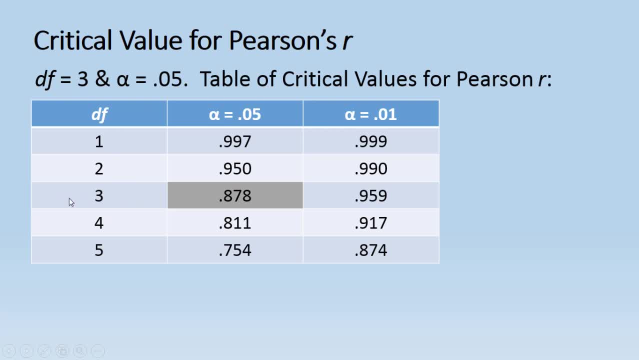 So we want to find the row df here of 3, where it intersects or meets with alpha 0.05.. So here the shaded value, critical value is 0.878.. So here this is the setup for hypothesis testing. 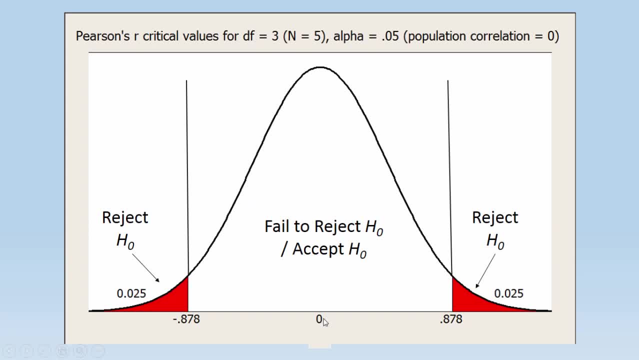 Now, here we have Pearson's R, the center is 0.. And notice the critical value. Remember we had 0.878, so I have a positive 0.878 here, a negative 0.878 here. These are my critical values. 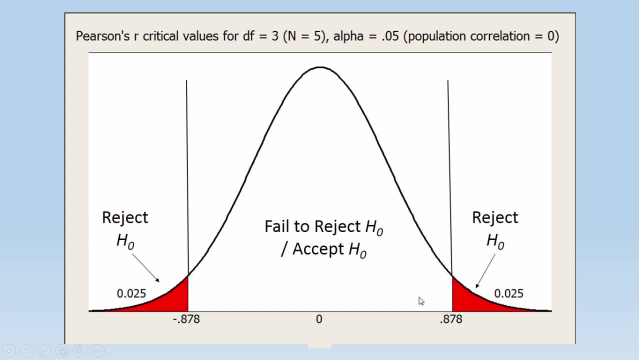 You can think of them as lines in the sand. Now, if I cross the critical value, if my calculated correlation is beyond this line in the sand towards the more extreme value here, or beyond this line in the sand towards the more extreme value here, then I will reject the null hypothesis. 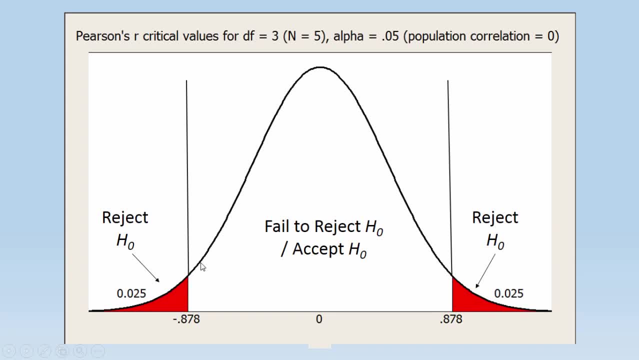 Either of these two values if I get it over to the right in the tail or to the left in the tail. So if it's bigger than 0.878, I reject If it's smaller or a negative value here. so if it's to the tail here, then I reject as well. 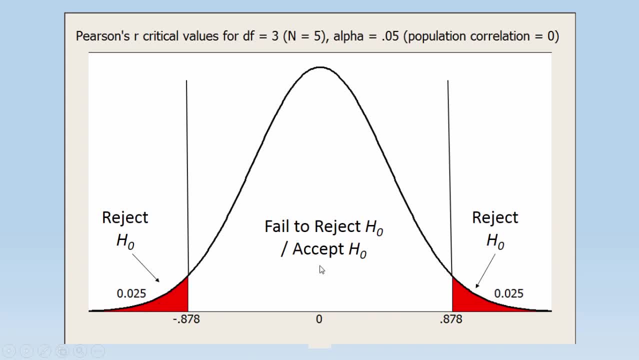 But if it's anywhere inside here, then I would fail to reject the null, or some people refer to it as accept the null. Now, our value, as you recall, was negative 0.9.. So it was right about over here somewhere in this area. 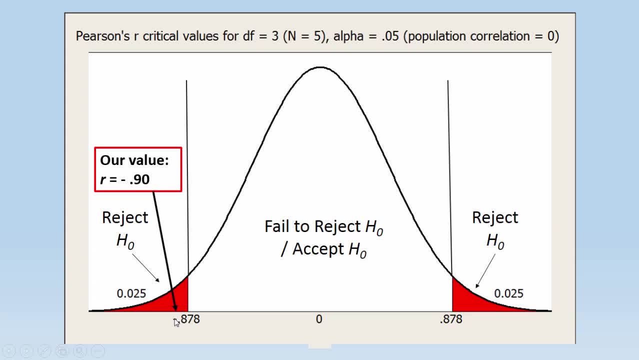 Notice: it's beyond that line in the sand right. If we have, for example, negative 0.88,, negative 0.89,, negative 0.9, we're in the tail here. So because our value was in the tail, it was beyond the critical value. 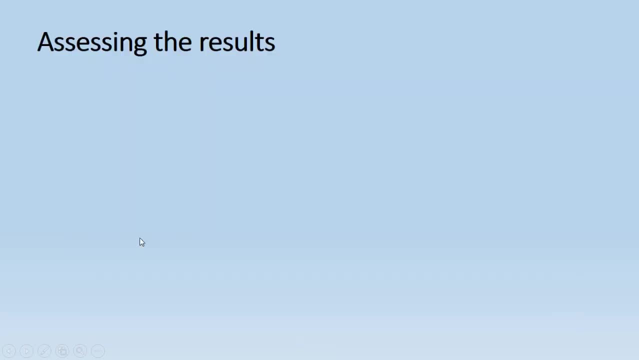 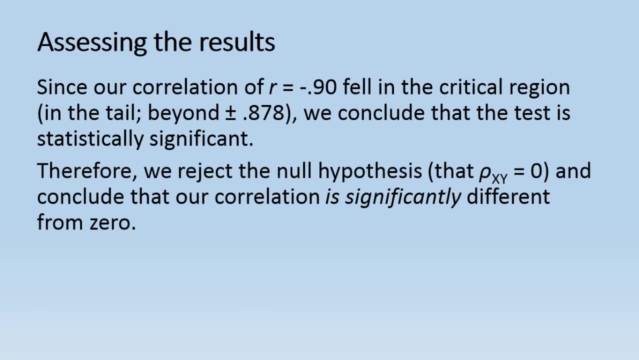 we're going to go ahead and reject the null hypothesis And when we do that, we conclude that the test is statistically significant. Therefore, we reject the null hypothesis- and- recall, we stated this at the beginning of the presentation- where the null hypothesis is the null hypothesis. 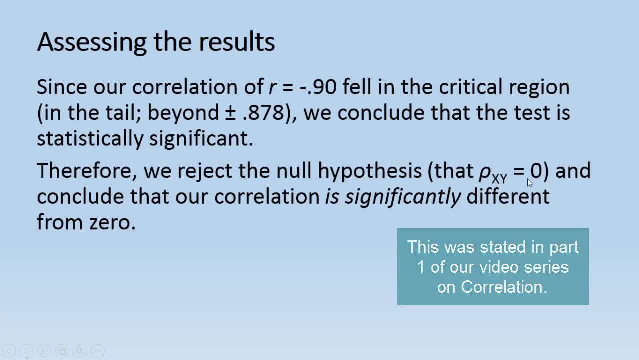 The null said rho xy equals 0, so we are rejecting that. And if we're rejecting that, then that means we're saying that rho xy does not equal 0. And because of that we conclude that our correlation is significantly different from 0,. 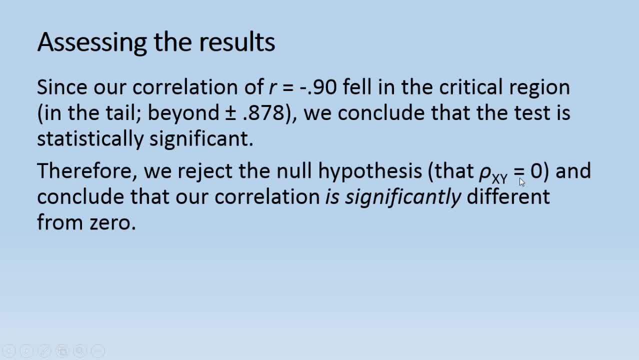 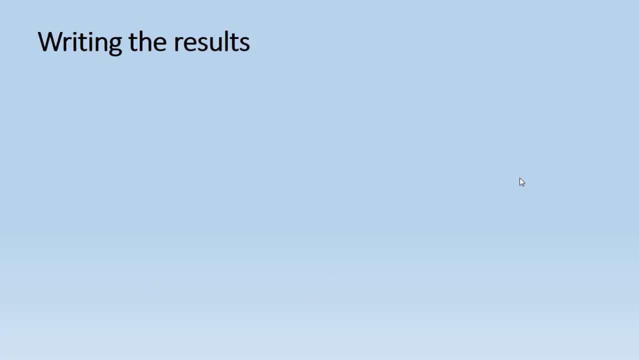 because we rejected this statement when our value fell in the tail, beyond the critical value or that line in the sand. And we can go ahead and write the results as follows: There was a significant negative. There was a significant negative relationship between x and y. 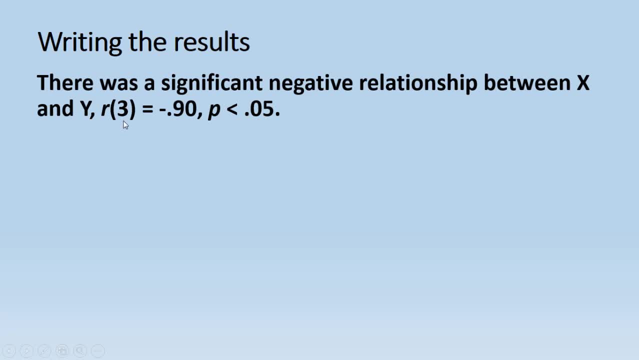 And then here we have r of 3,- and this is the degrees of freedom- equals 0.90, that's the value we calculated by hand, and then p is less than 0.05.. And in these results, as I said, 3 is for the degrees of freedom. 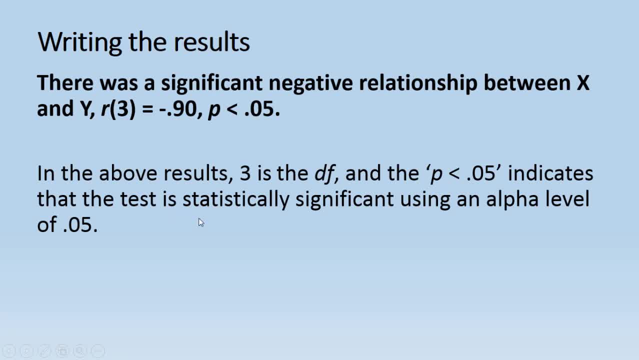 The p is less than 0.05 indicates that the test is statistically significant using an alpha level of 0.05.. Now, if the result was not significant, say that we had a correlation of negative 0.80.. And recall the critical value was negative 0.878.. 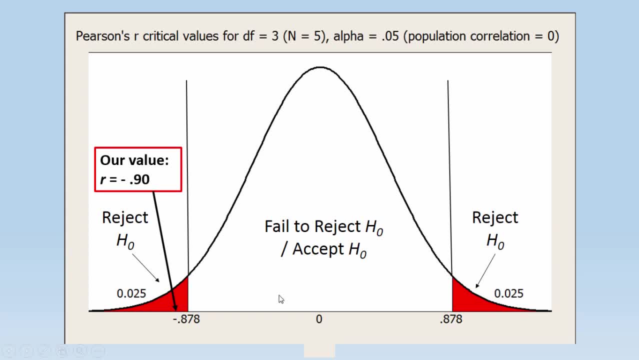 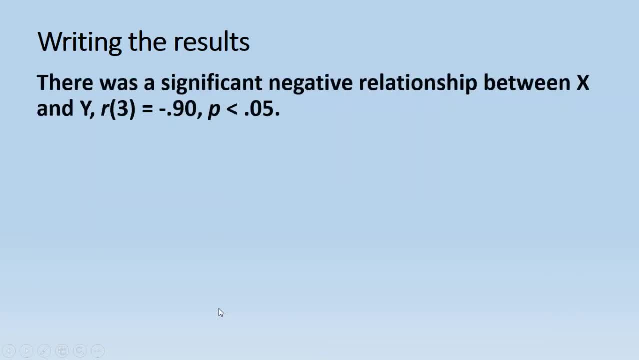 So 0.80 would have been about right here. It would not have crossed that line in the sand. If that was the case, then we would have said p is greater than 0.05.. And we would have said there was not a significant negative relationship between x and y. 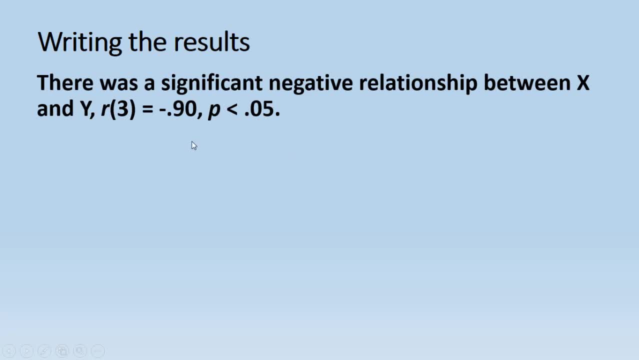 But because it was significant, we do go ahead and write it, as was shown here, and we write: p is less than 0.05.. So anytime you have a result that is statistically significant or beyond that line in the sand, in our distribution, in the tail,